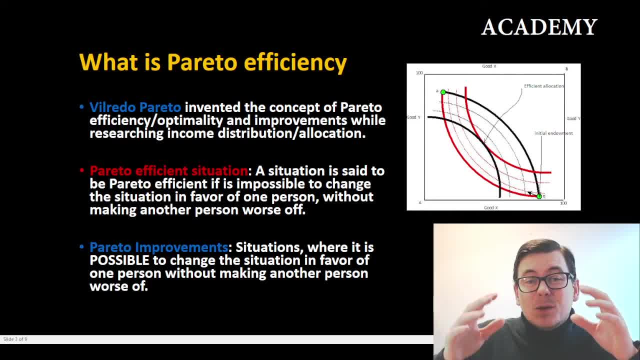 When we reach such a status we say that we are in a Pareto efficient situation. So we can see it up here from the Edgeworth box, from microeconomics, that when we have two indifferent curves hitting each other and we cannot move any further without the other parties. 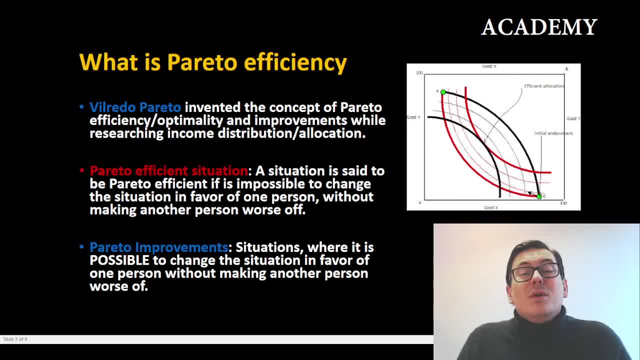 indifferent curves, kind of move back. well then, we are in the Pareto efficient situation. But to get there- and this is actually the most interesting part, because to get to that point where we really want to be, we can, on the way, make Pareto improvements. And these are the 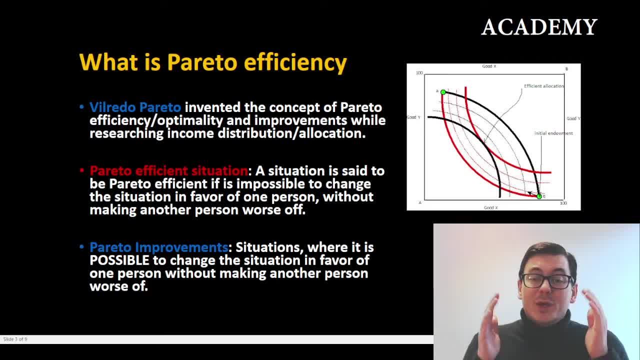 situations where we can actually make Pareto improvements, And these are the situations where we actually can improve the relationship between, let's say, two parties, where we improve one's wealth or value without hurting the other party. If that is possible, we should do it because it. 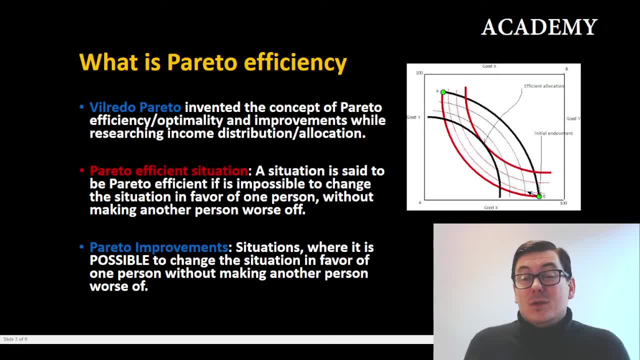 increases the value of the relationship, and that is good in terms of economics. And by doing this we're talking that we're making a Pareto improvement, we're improving the relationship between the parties, And that's what we're talking about here. We're making a Pareto improvement. We're improving the relationship between the parties. 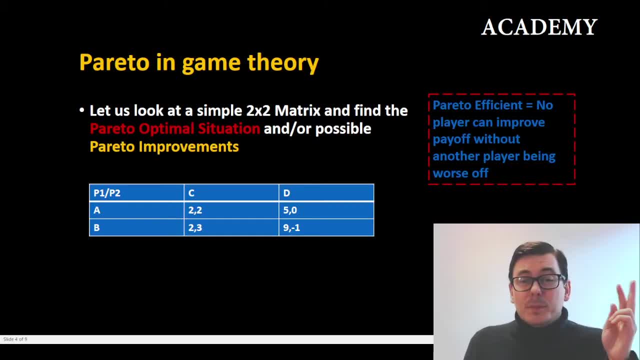 So let's put it into game theory. I put up a two by two matrix kind of translated the efficiency term up here to saying: Pareto, efficient equals no player can improve payoff without another player being worse off. So we have two players Each of. 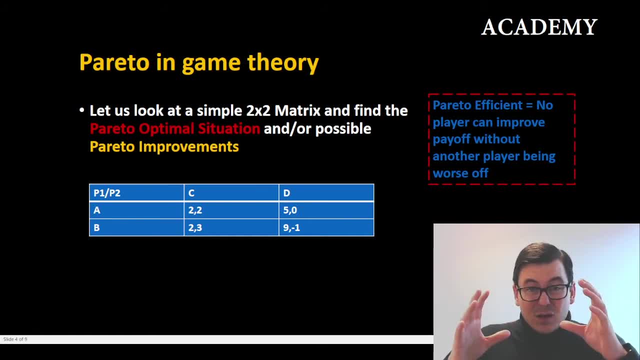 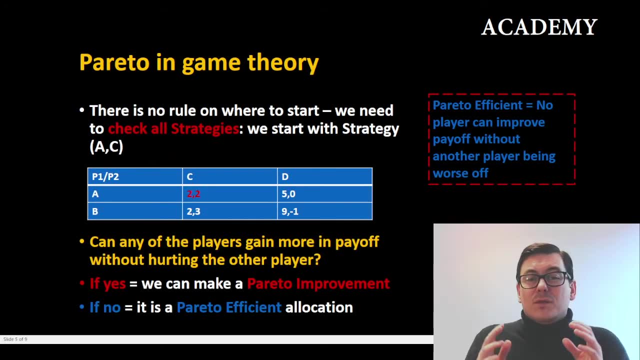 them have two strategies. We have a set of strategies that gives certain payoffs to each party. Let's start the analysis. We can just start from the strategy AC, because there is rule of where to start, because we need to analyze all four conditions. So in AC, 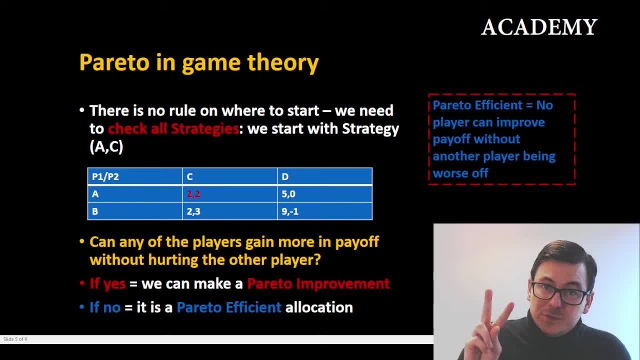 each party will get a payoff of two. What we should ask ourselves now is what I highlighted in yellow: Can any of the players gain more in payoff without hurting the other players payoff? If the answer to that question is yes, then we can make a Pareto improvement and we should thrive to do so. If the answer is: 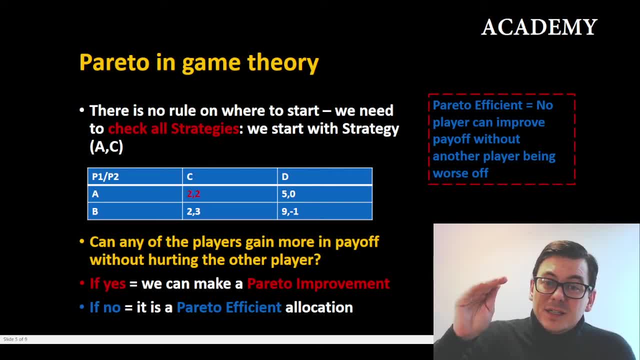 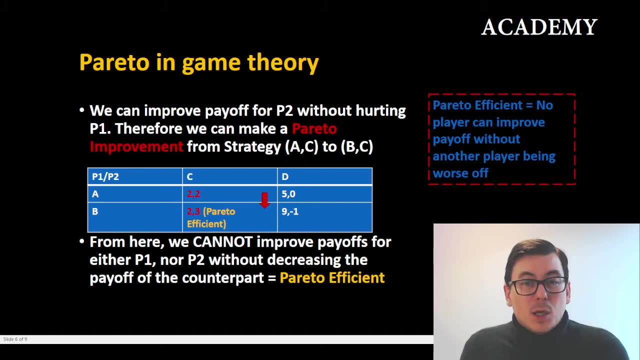 no, then we are at a Pareto efficient level and there's nowhere else to go, Not in terms of Pareto efficiency. So let's look at it, because we can see that in strategy BC, player 1 gets a payoff of 2 and player 2 gets a payoff of 3.. So we 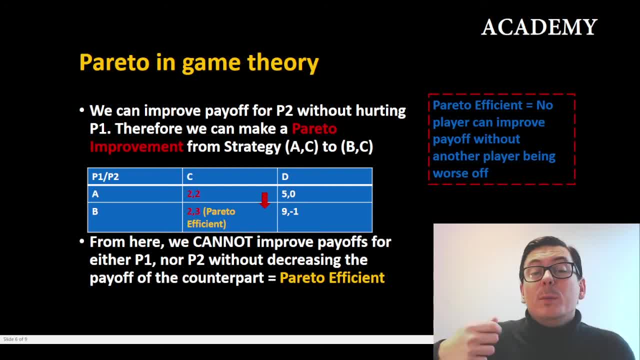 can see that in strategy BC player 1 gets a payoff of 2 and player 2 gets a payoff of 3. So we can actually here make a Pareto improvement if we move from AC to BC, because here player 2 will get one more in payoff without hurting. 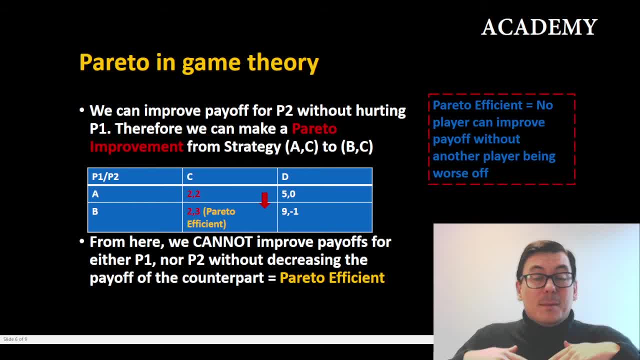 player 1.. So here we can make a Pareto improvement which we should thrive for to do. Can we make more improvements from here? So now we are at BC giving 2.3 and we can see if we move to AD it would be 5.0, which means that player 2 will. 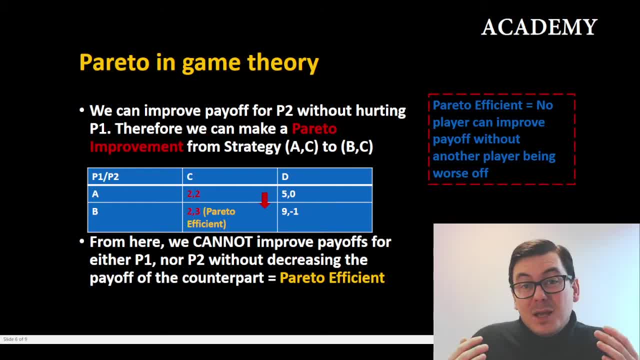 go down and player 1 will go up. and the same account for strategy BD, where player 1 will get 9 and player 2 would get minus 1. So we cannot really make anymore Pareto improvements. Hence we are at a Pareto efficient level. 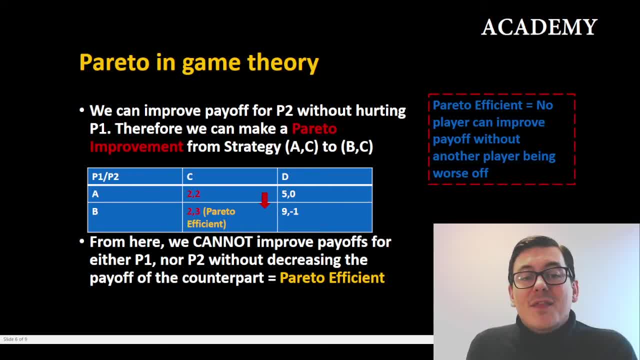 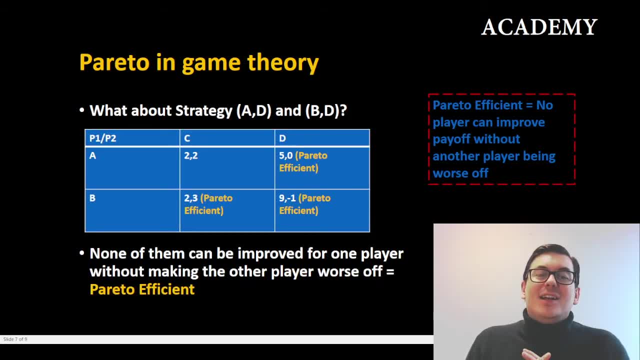 So we can now state that strategy BC is Pareto efficient. We should thrive to achieve more bidding results and to bring India himity efficient. now we'll look at the two last outcomes, and that is ad and bd. i already put out the results here, because it is very clear that ad gives player one five, player two zero. we cannot. 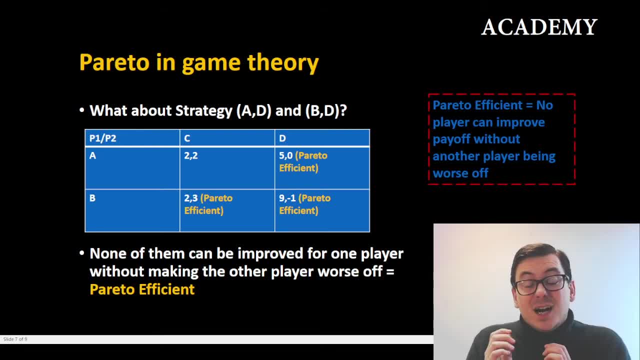 move anywhere without hurting either player one or player two. therefore it is also a Pareto efficient strategy and the same accounts for strategy bd. so in this game there's actually only one strategy that does not equal a Pareto efficient status, and that is strategy ac. so we have to remember when we're talking about efficiency. everyone says efficiency all around.